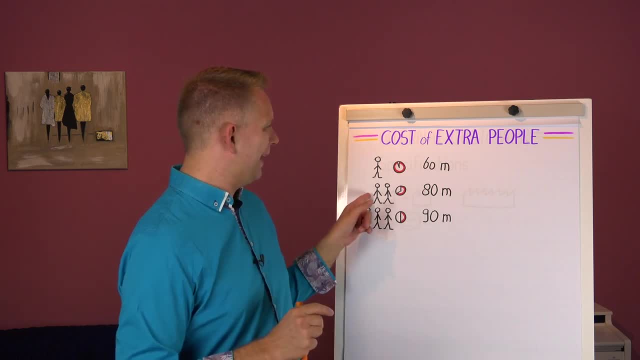 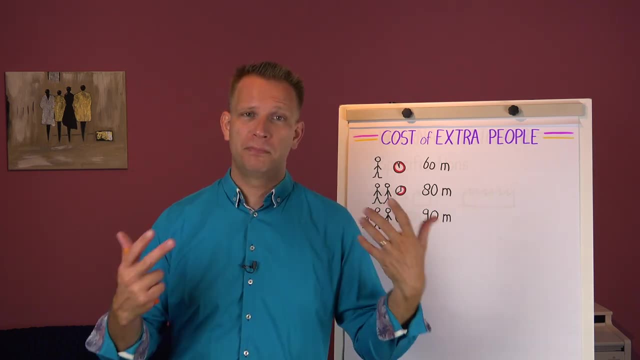 Now, how about we put two people there and the cleaning time it goes from 60 minutes to 40 minutes. We do, of course, have two people there, so the man-hours increase And most companies will tell me if you're going to put an extra person at that line. 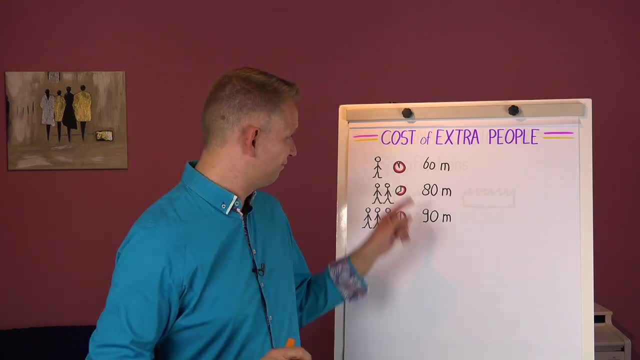 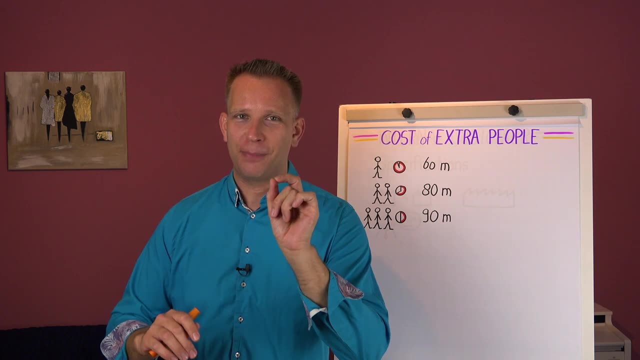 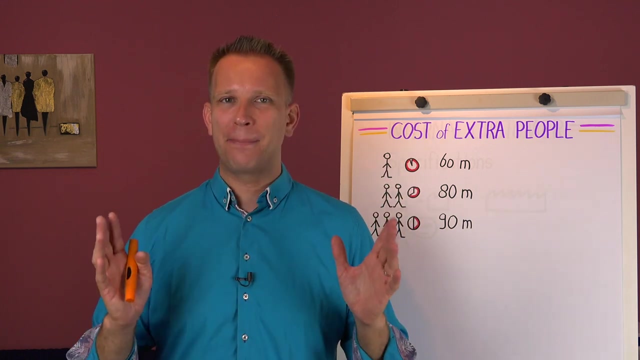 around the clock just to save 20 minutes. it's ridiculous. I say no, no, no. This extra person doesn't go there around the clock. We're not talking about adding an entire extra operator. Can you, during the cleaning, get somebody else there? 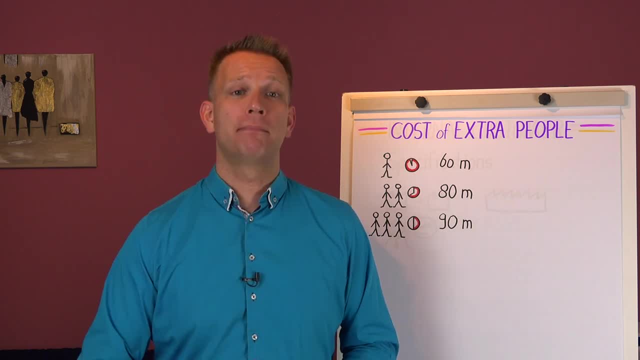 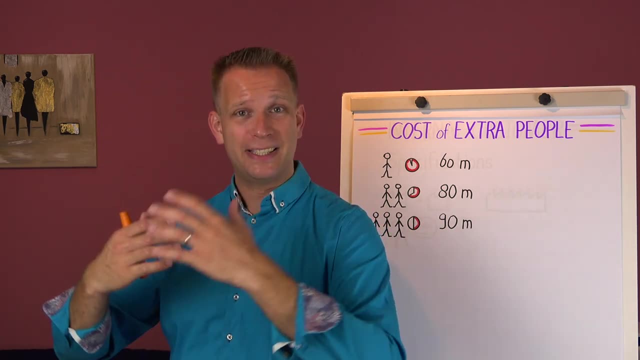 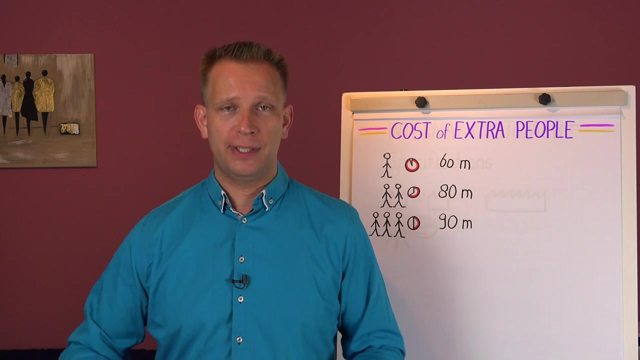 to help with the cleaning. Maybe the supervisor can do this. Maybe you have a different department, for instance the assembly department, that can send somebody over. You don't. You don't have to train them fully as an operator. You have to train those people then to be able to clean or do specific tasks during the cleaning. 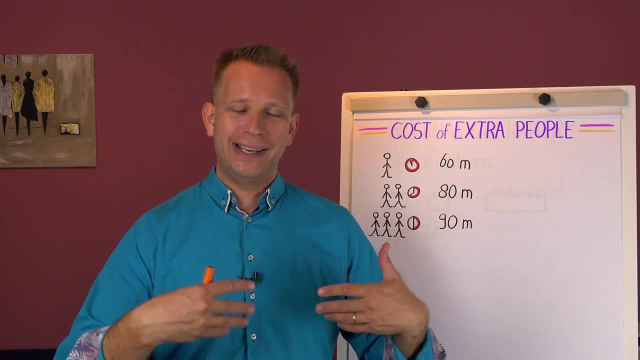 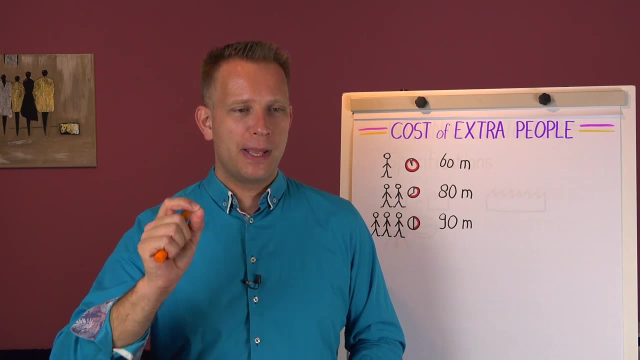 as long as they help that main operator with the tasks, that they can become quicker. It's difficult to plan- I know it is, But it is definitely possible. But then we get to this next thing: If we have two people that each spend 40 minutes there, 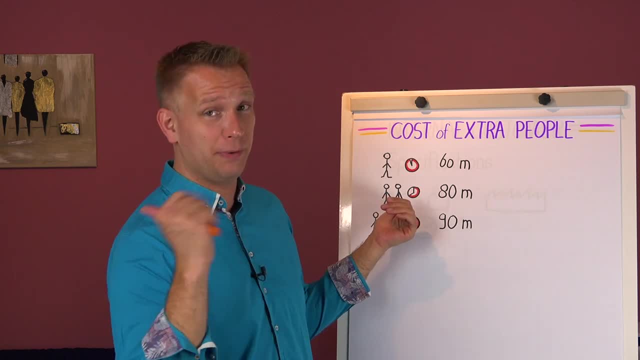 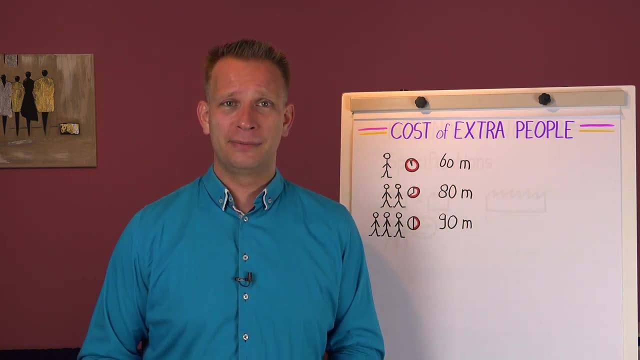 and probably that second. one has to spend 15 minutes getting over 15 minutes getting back to their old job, so they're even spending a bit more time, but we're spending at least 80 minutes there, So we're not saving time at all, right. 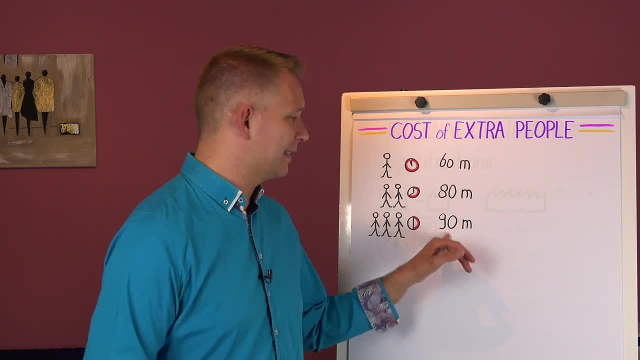 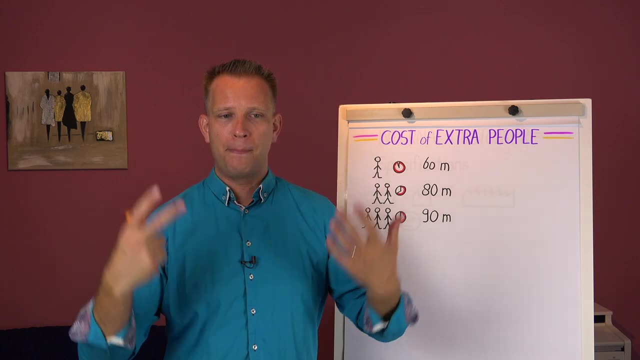 Or I say: well, let's go for three people and we'll do it in half an hour. It's 90 minutes, It's even worse. But think of the rest of the line, Think of the benefits that might be there. 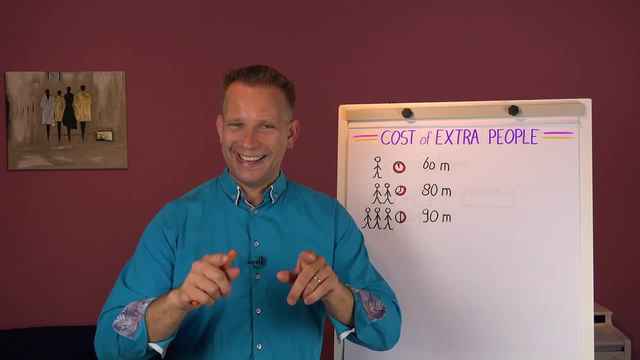 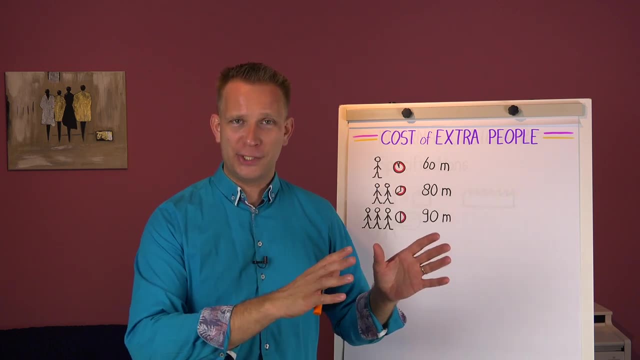 Now there is this wonderful little film. I will also link it on YouTube so you can see the whole thing, But it is about a comparison of the Indy 500 and the Formula 1. And of course they had some rules back in the days. 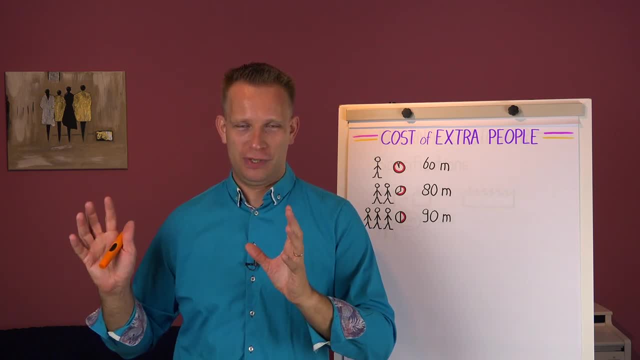 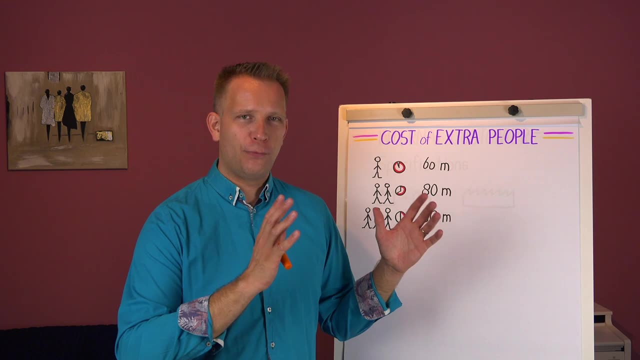 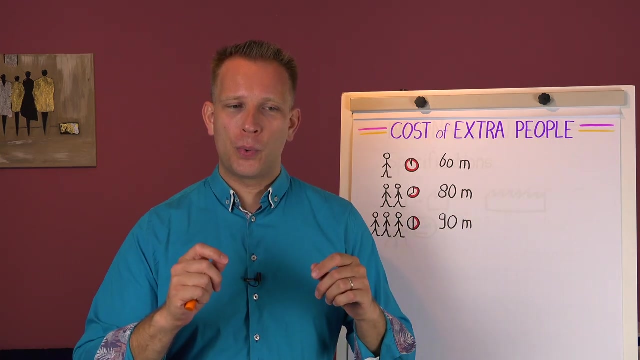 But you see how cringingly long it takes to change over that Indy 500 car in the pit stop And then this Formula 1 pit stop team that does it in. well, I won't spoil it, but a lot faster Now that Formula 1 team. they had 23 people standing around it. 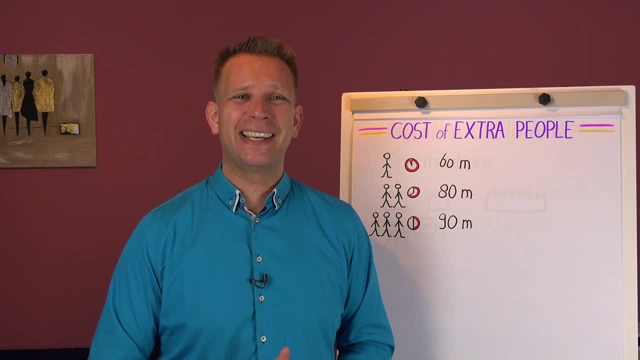 In 500, only four, Twenty-three people standing. They're working, They're working, They're waiting most of the race just to do those couple of seconds of work. Are they completely crazy at the Ferrari team? No, they are not. 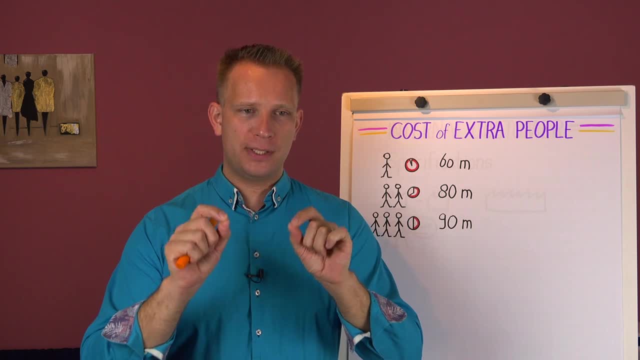 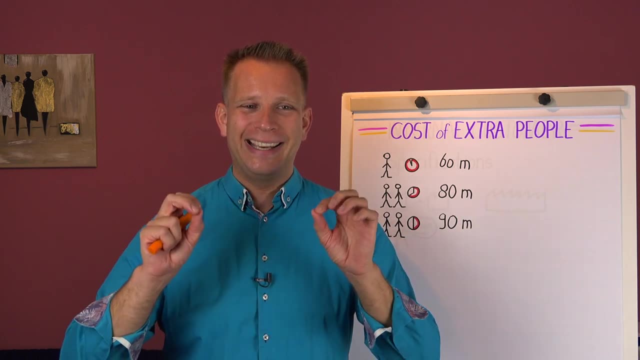 They know that even shaving off those last tenths of seconds in a pit stop is going to be the difference between winning a race or not. And that difference- winning a race or being number two- is a difference of a million dollars or something like that. 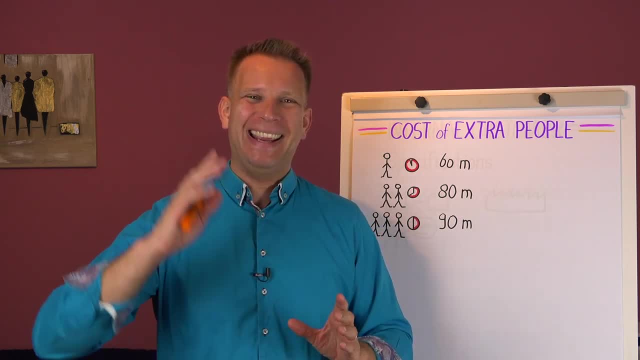 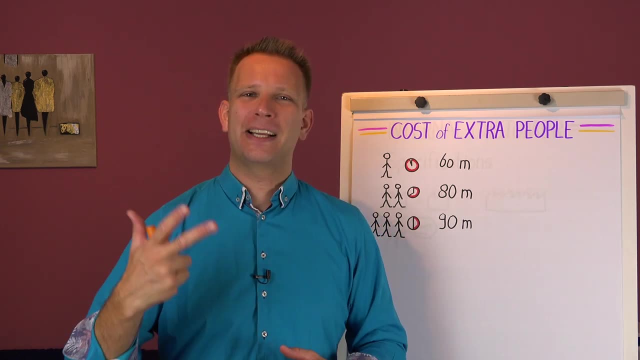 So they know, They know, They know that they will get this money back in droves, And that's why this is such a wonderful little video: to really repeat it a couple of times. First, look at it yourself, but repeat it a couple of times with your colleagues. 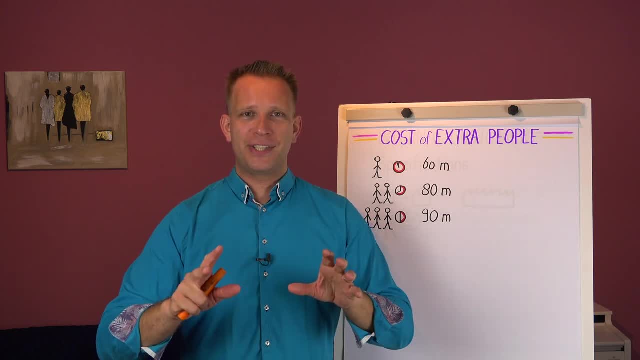 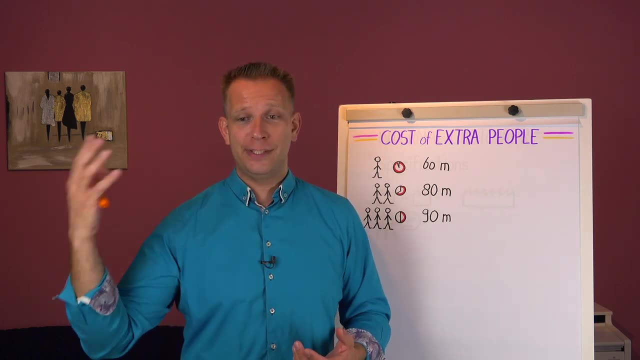 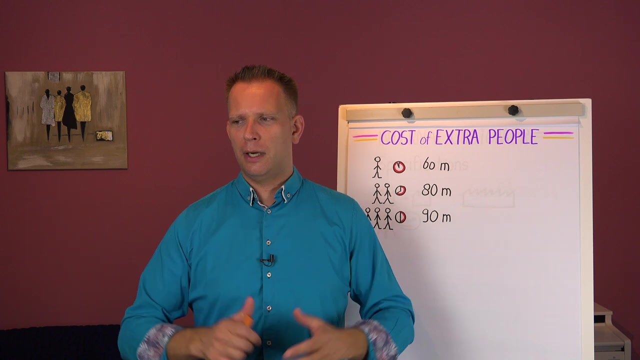 Because all of the problems they see you can probably explain, You can probably use as a wonderful way. So when I show this video to people in production maintenance at companies all over, I get all kinds of. But the technology has improved. 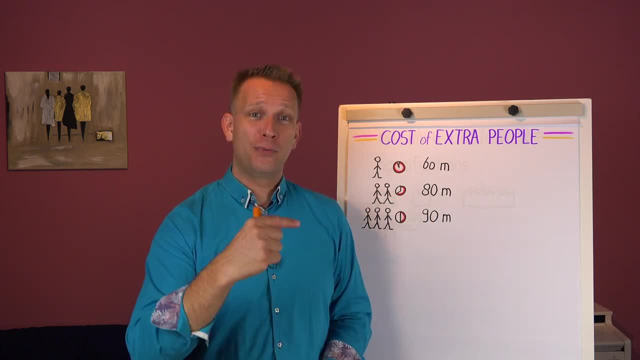 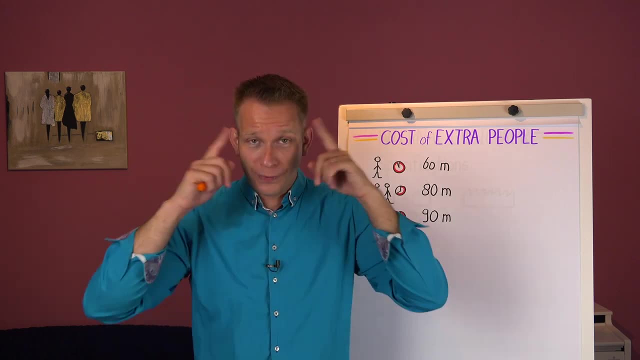 Okay, so what technology would you need to improve the efficiency of the cleaning at our factory? They have so many more people, Okay, so where can you get the people from? Ah, that's very expensive. Do you think that Ferrari has so many people because they have too much money? 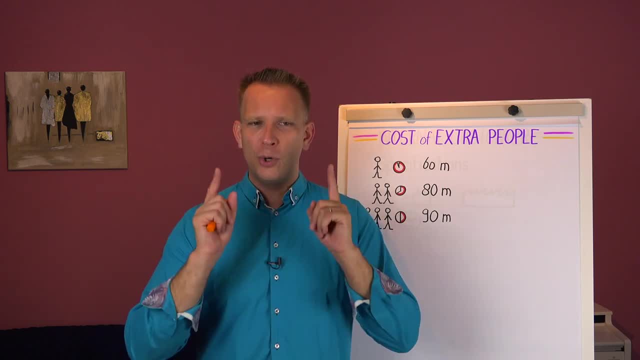 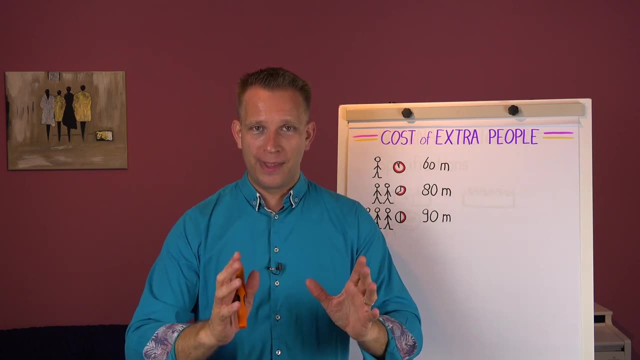 Or is it a real economic choice? What is the goal? The only goal of them in that race is to become number one. That is the million-dollar goal. So you can spend, You know, even a couple hundred thousand to make sure you get there. 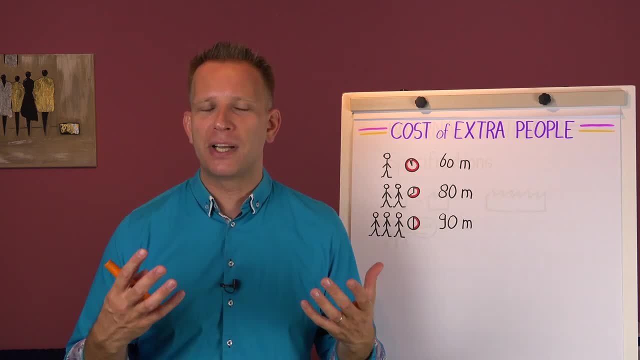 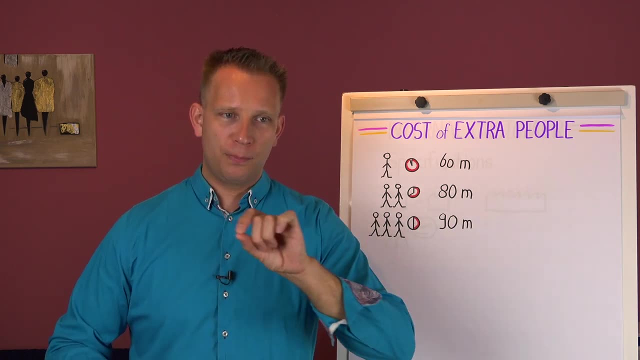 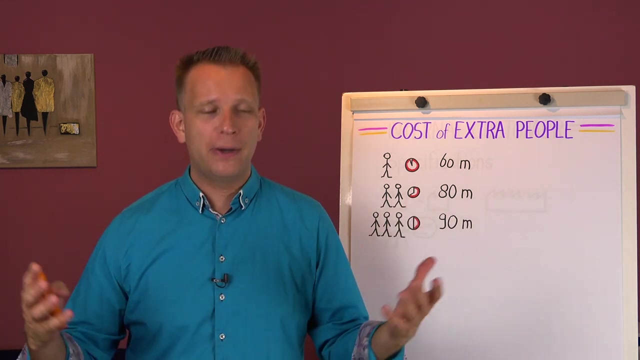 And then they start seeing it, And especially maintenance guys, They will say, oh yeah, but that's gold-plated maintenance. Well, if your lines and your processes are bringing in a lot of money, you can spend more on maintenance. Now I will say this: one line that runs for two odd shifts in a week. 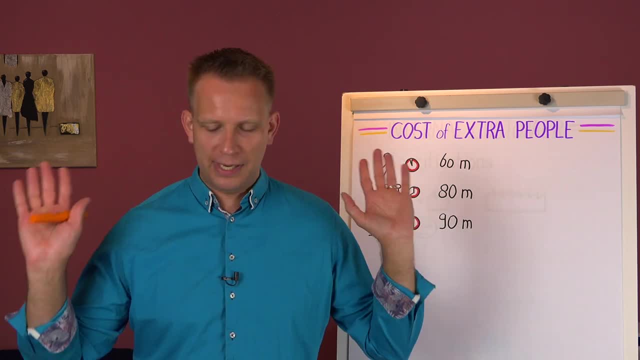 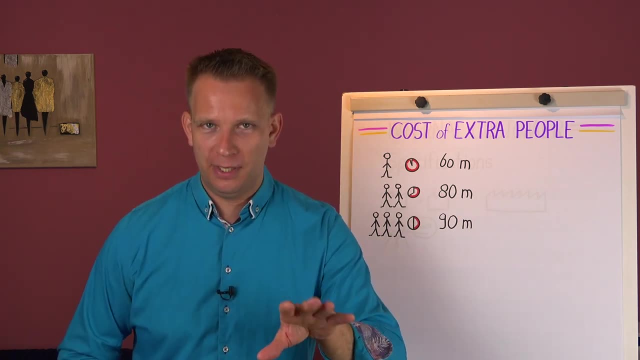 You got plenty of time to do all kinds of maintenance before and after that And you can also- you know, if a production run fails, just do it again tomorrow. That line does not deserve Formula One-type pit stops. But your critical line that is already capacity-constrained. 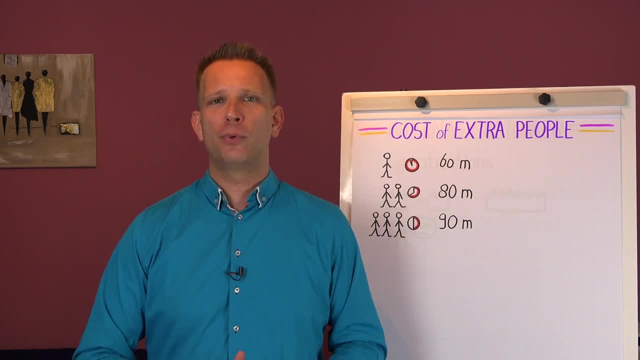 that already runs 24-7, and that actually has even more market demand. if you can squeeze out some extra production there, that is going to generate a lot of money, And let your finance team help you with that. how much money it actually is. 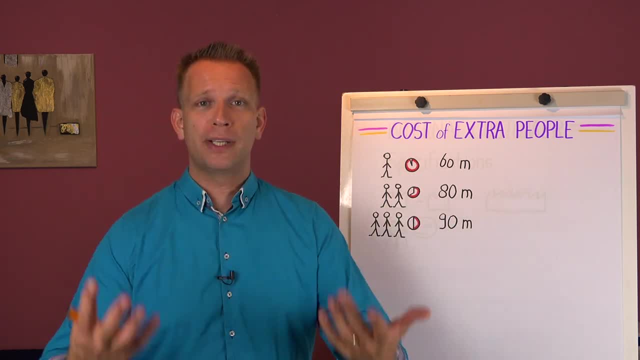 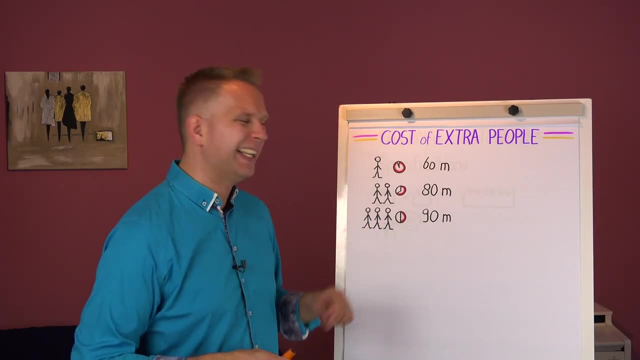 But you will see that spending, if you spend a bit more time during a cleaning, during a changeover, it's going to be no problem. They are all in favor of it. It just requires flexibility from your production team, from your personnel planning, so to say. 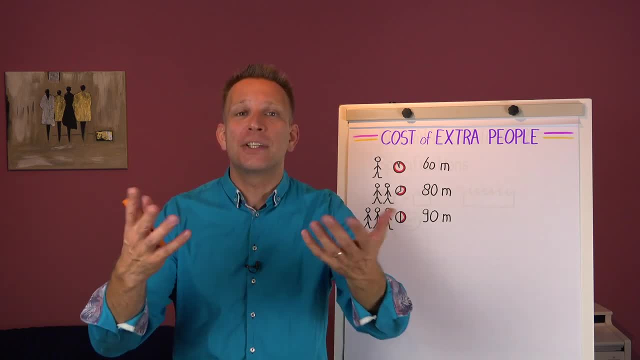 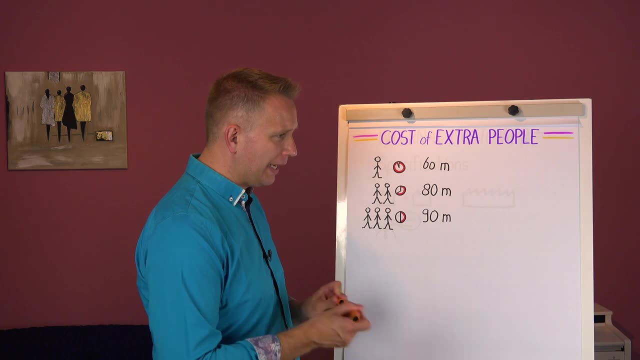 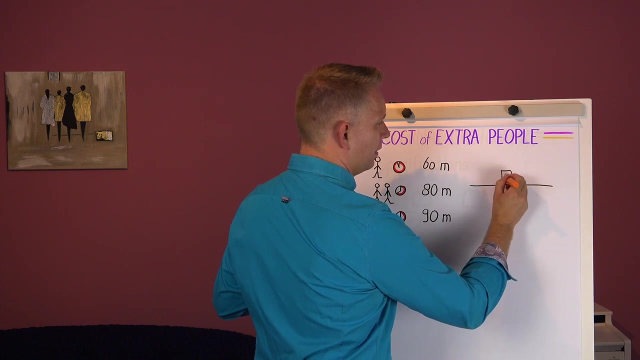 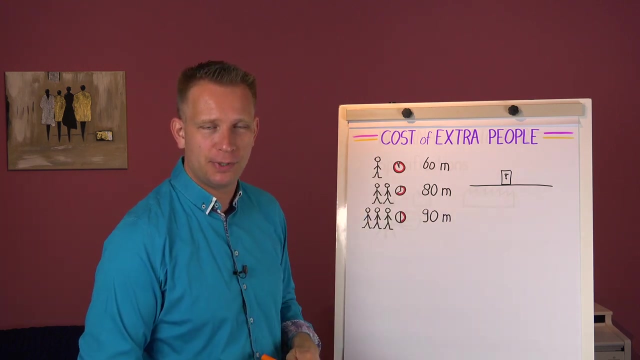 It requires you to organize yourself better, But hey, that is what's going to give you a competitive edge. So what if we have a line and when we check the total line, our machine is the bottleneck. The rest of the line can do all their stuff in about 15 minutes or so. 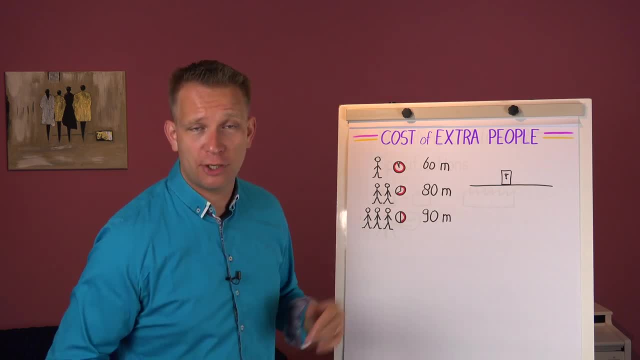 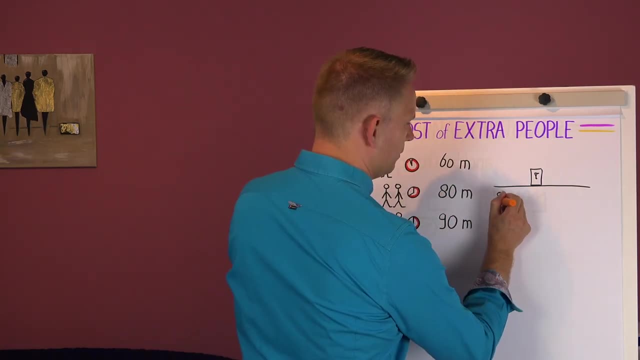 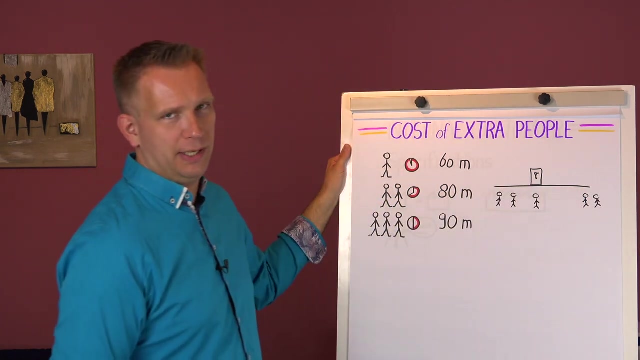 They can get everything changed over. It's mostly manual stuff or it doesn't really need so much cleaning or whatever. So we've got the bottleneck here with the cleaning. Very simple example. I don't even assume that the product goes bad or we really need the extra output. 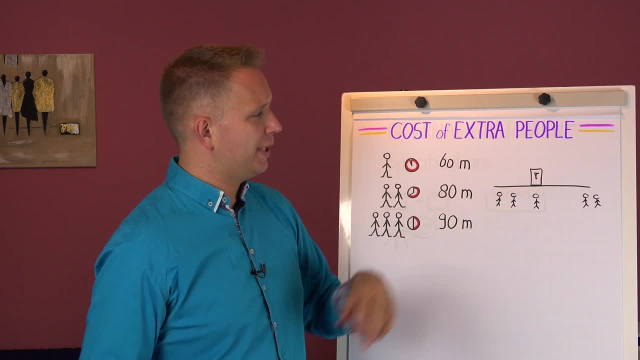 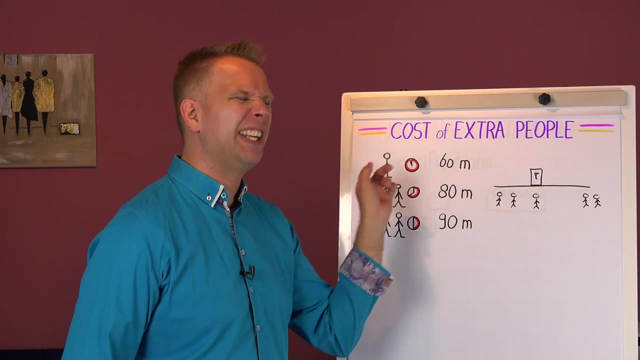 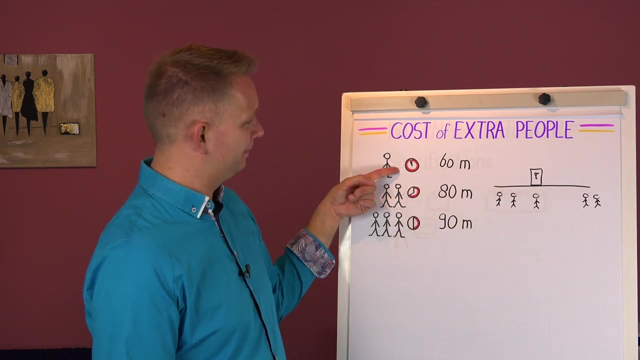 We just have a line where there's a couple of machines around it, a bit of assembly and packaging And on the total line. so I'm not talking about this machine that we're cleaning- the total line has five people. So we've got five people times 60 minutes. 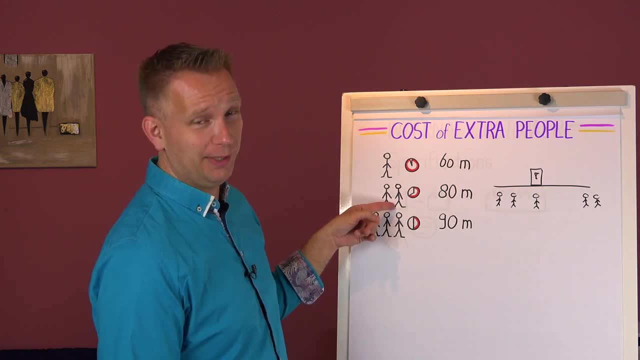 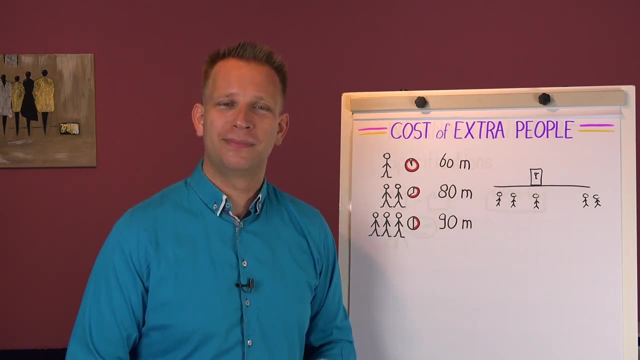 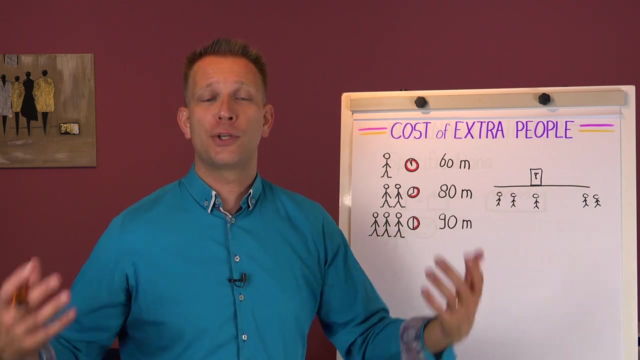 or six people times 40, or seven people times 30. Hey, Actually, our total time is going down Interesting, eh So, by spending a bit more because we reduce everybody's time, since this is a bottleneck, it's already great. 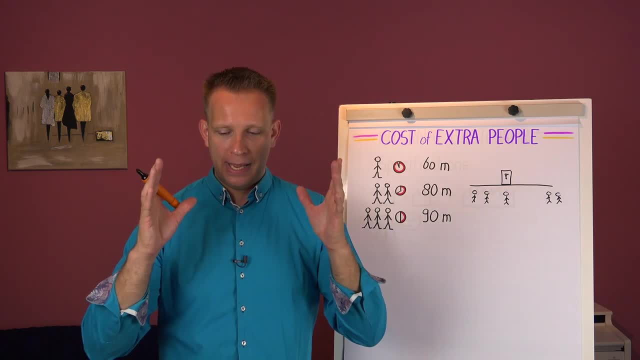 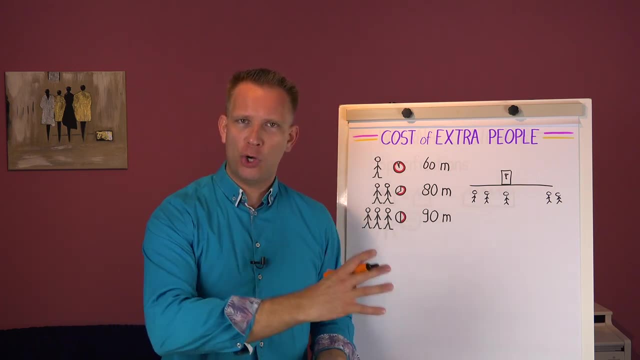 But now let me discuss a practical example where we did this, and this was in a whey drying tower. Now whey is that liquid that comes off cheese, But whey has a lot of sugar in it- still lactose from the milk. 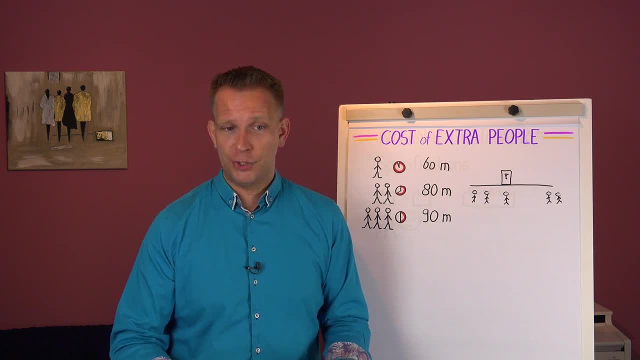 It also has the bacteria in it that are used to make the cheese. So this is a very bioactive substance, And when you make cheese you get whey as well. You need to do something with the whey. It's not even allowed to just flush it down the drain in most countries. 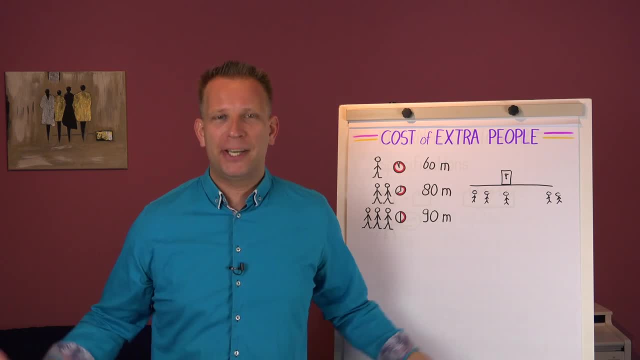 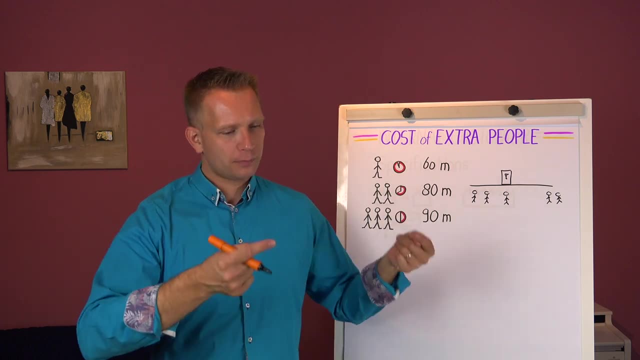 because there is so much, you know, organic matter in there. But apart from that, it's a waste because it's a nice material. Now we had this on-site whey drying tower and it would first concentrate the liquid whey. then really thicken it up into almost sort of a paste that would go through the spray dryer, The spray dryer when cleaning it, which was needed every about one, one and a half days with that tower and for those in the industry. yes, I know that was a lot. 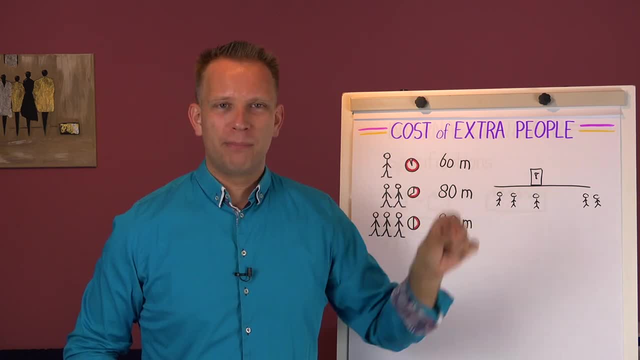 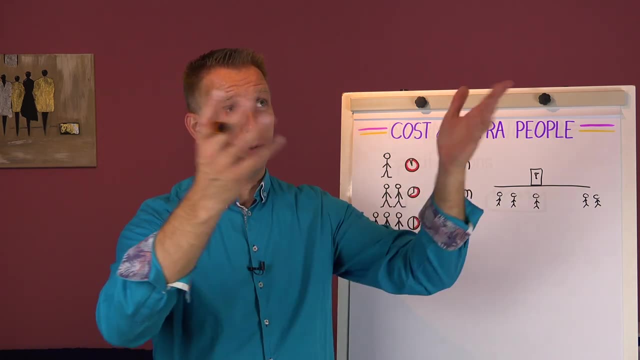 but with an old anhydrous tower we would spend about two hours to clean it. A lot of manual work all around it. You need to cool down the tower a bit and then do all kinds of things inside as well, And there is some piping around it. 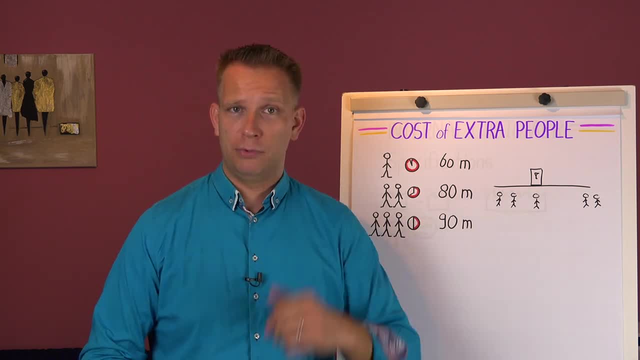 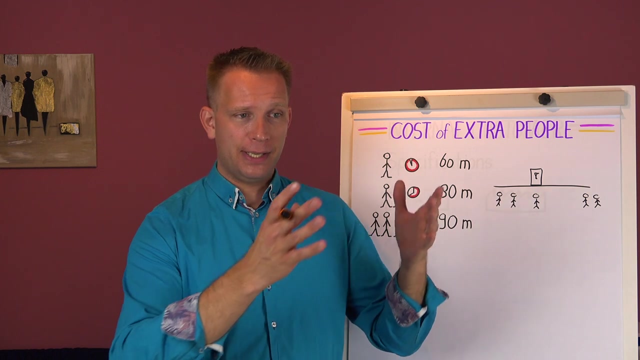 So there is a whole bunch of different things that needed to be cleaned, And it was one operator doing that. We then had trouble with the capacity of this line. We needed to clean it well, but also get it done, because actually what was happening is that 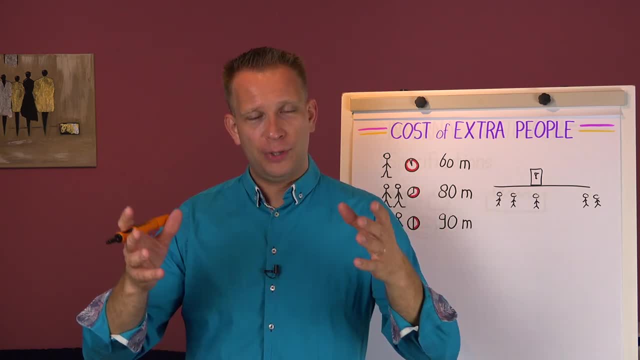 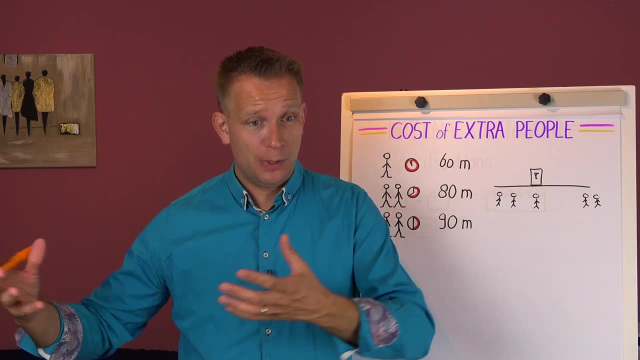 during the time that we were cleaning this sort of concentrated whey, and the fresh whey as well. they were all acidifying, And when we were at the peak of cheese production, we had more whey almost than we could dry, So this was all acidifying. 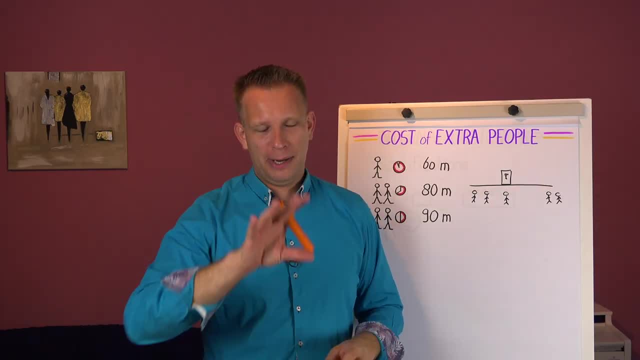 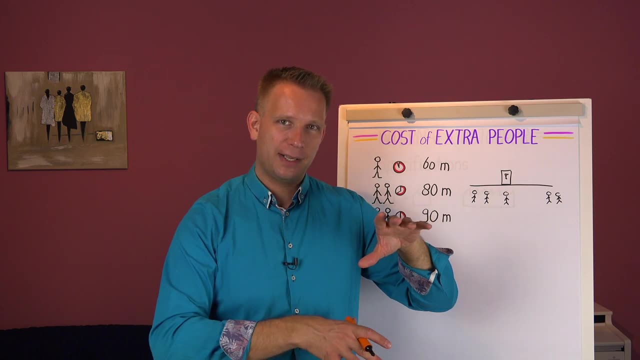 And as soon as it becomes acid you cannot really dry it anymore. I did make a video on this before, where we also went to sell, but this is a really lower cost, but selling a part based on the predictions, just to get rid of this over acidification. 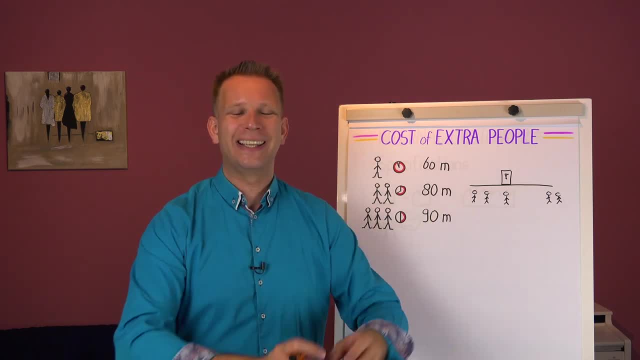 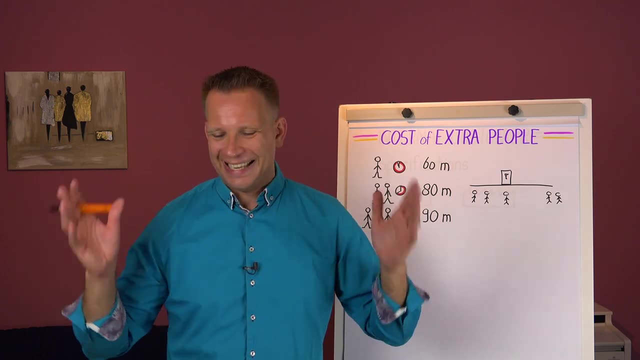 But the other thing we did was we made sure we could clean a lot faster And we discovered that a couple of things could be prepped in advance, But you just need to clean when the tower is down. But what we did is we got in two people. 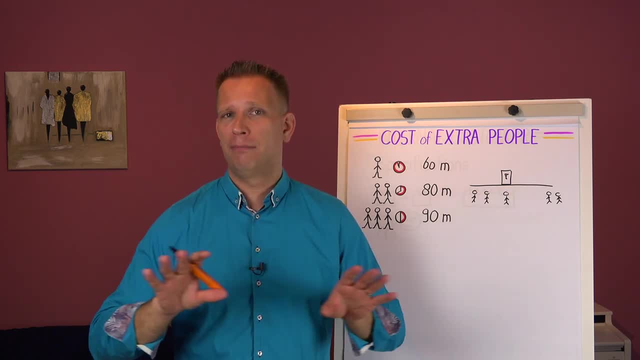 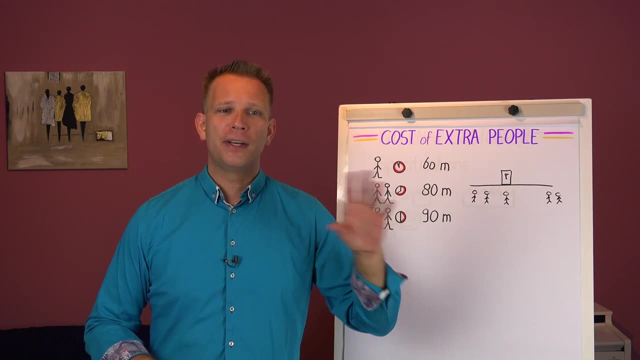 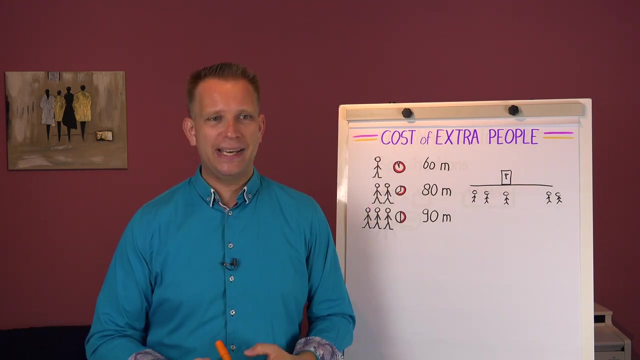 from a totally different department. They were not the drying tower operators at all. They would normally not even work in the same department. They were just operators that worked in a totally different department. But I mean, they are trained as operators. They have a basic understanding of machinery. 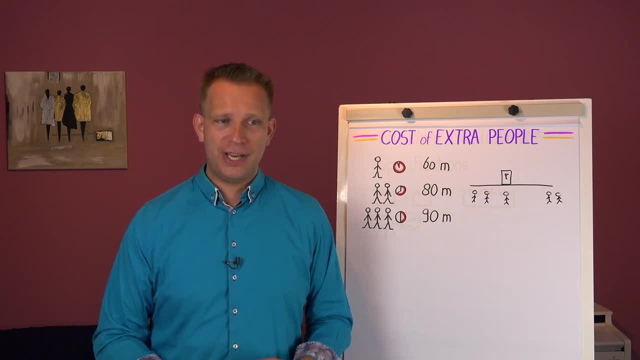 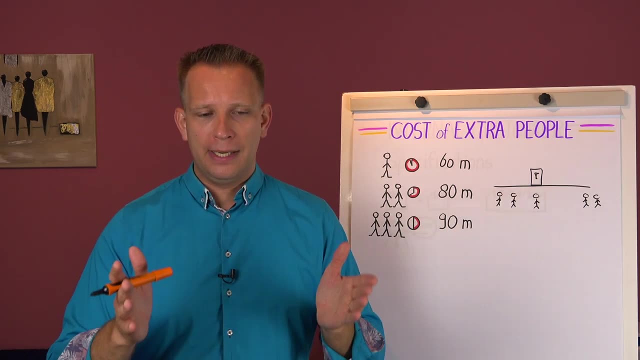 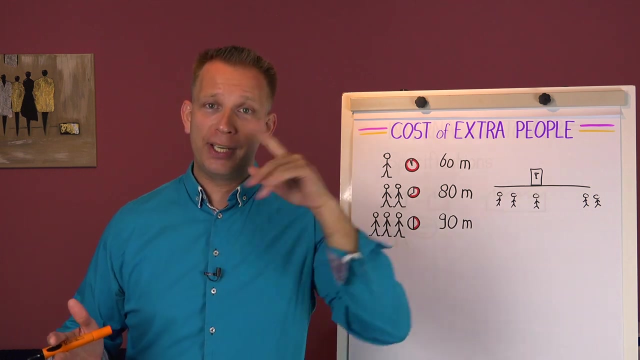 and how things work And we could quickly teach them how to do specific cleaning tasks around this way, dryer And we would. just when it was about to go down for cleaning about 20 minutes before it would shut down, the operator would call the supervisor. 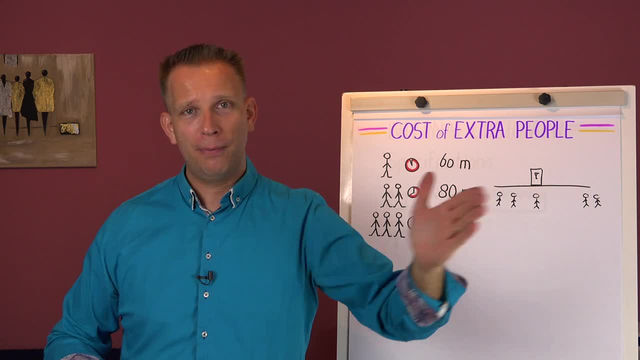 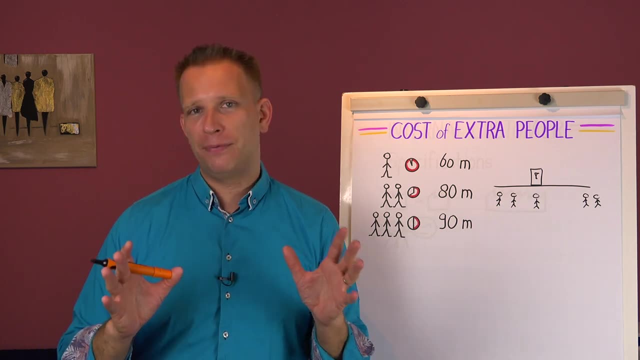 of the other department. They would free up the two people, They would move over And by that we can get the cleaning done in about 45, 50 minutes. So we definitely spent more people time on the cleaning, But we got over an hour back. 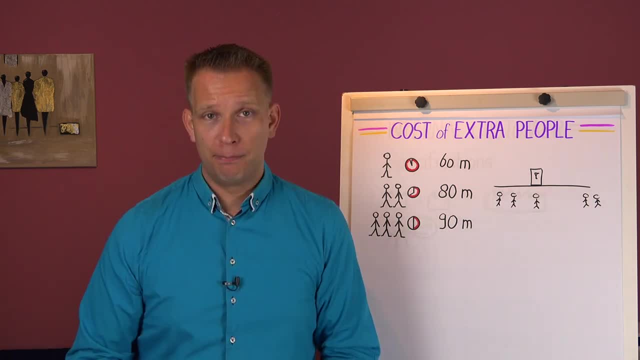 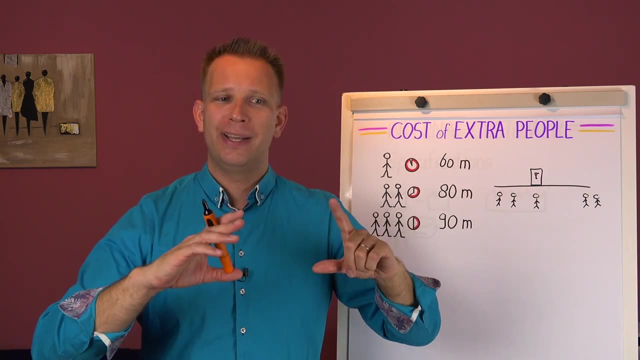 of cleaning each day, which is such a nice boost in productivity that we could actually get ahead of the way that needed to be dried, Because this snowballed into the way, being a bit fresher, meaning that it would dry much easier. the speed of the tower picking up. 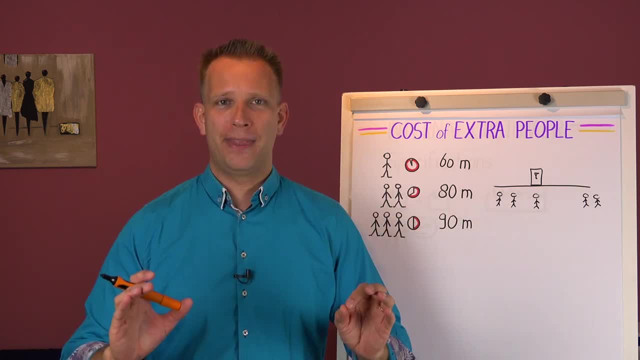 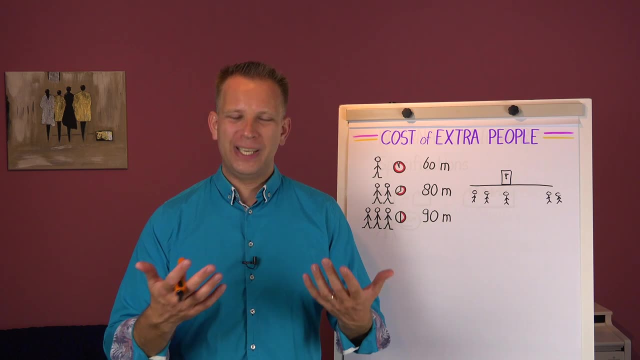 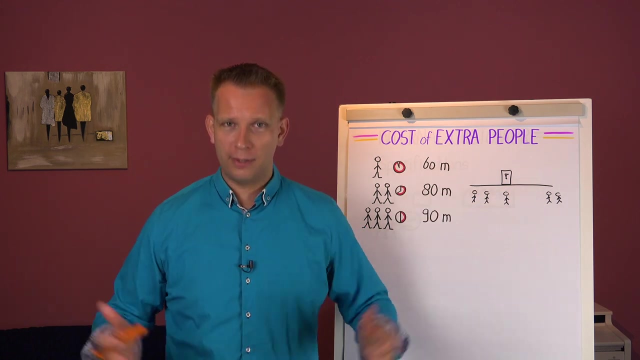 In the end that was just a win-win business case. It was wonderful Because we had, I would say, the courage to really change up the organization. We were drawing in people from a different department under a different manager. The one factory was the total factory goal. 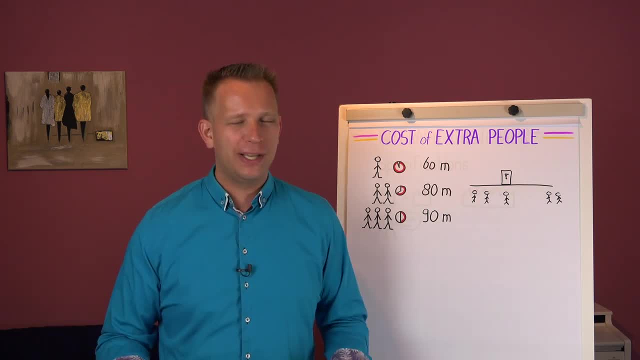 to make sure that everything is working That way. dryer did not need free operators there at any time. That would have been a waste of personnel, But during this high-intensity cleaning moment we did need them. So we trained them, We organized that they would go there. 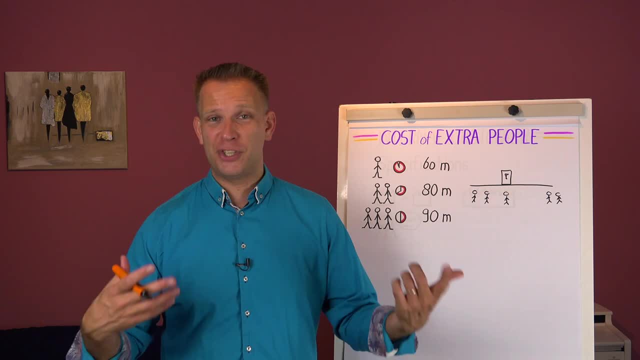 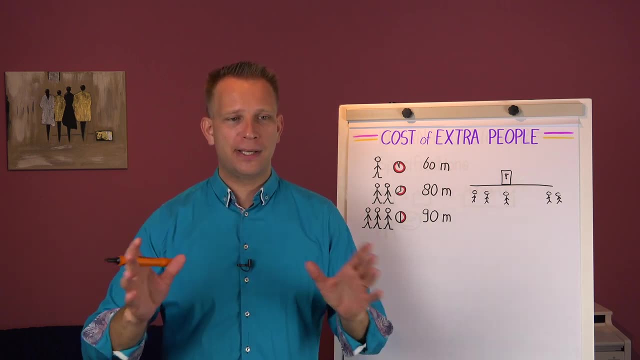 when needed. We didn't have a lot of such lines, so we could not make a dedicated cleaning team who would sort of go around the factory. No, these were just people that got a completely different task added on top of their normal work. 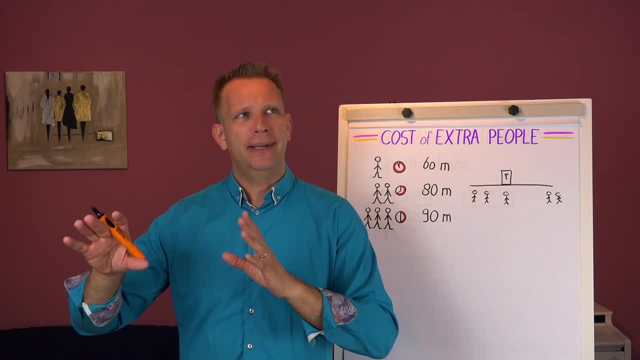 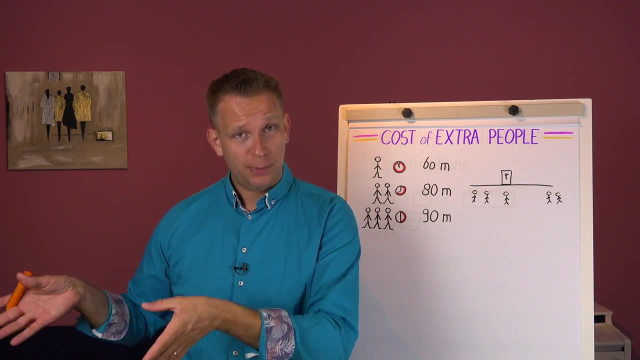 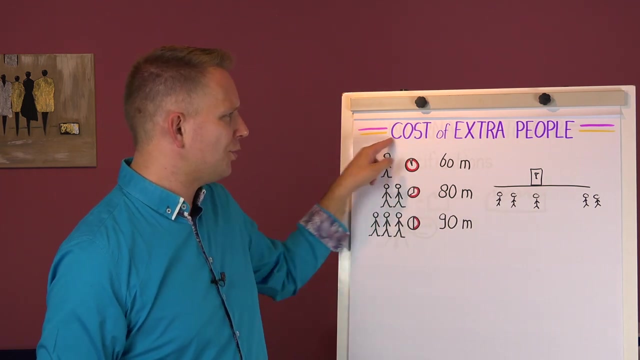 That work would stop for them. They had a couple of flexible lines and the process continued. But anyway, basically where they worked stopped for that hour, but it made the whole factory so much more efficient. So think about not just the cost of extra people.